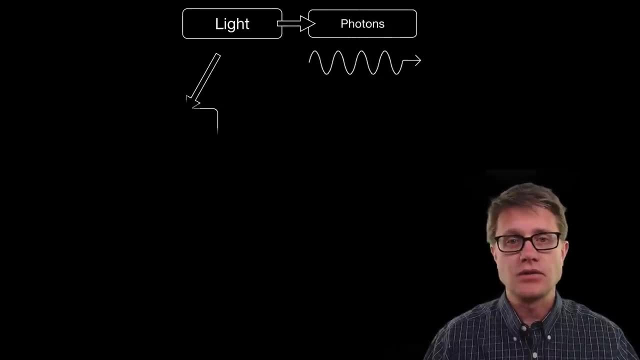 and a particle, And so light travels as photons And those photons can act as waves and particles. Evidence that showed us their waves is their interference. They can interfere with one another, Sometimes build up the waves, Sometimes build them down, And they also, if we look, 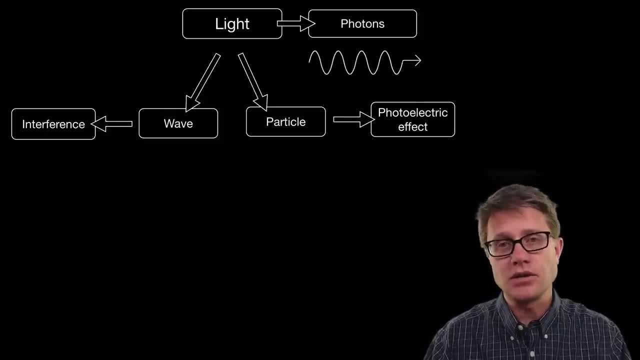 at them as a particle. the photoelectric effect tells us that photons are quantized. They travel in these discrete units like particles, And so if you are a physics student or a physics physicist, how do you know which model to use? Well, it really depends on a sense of 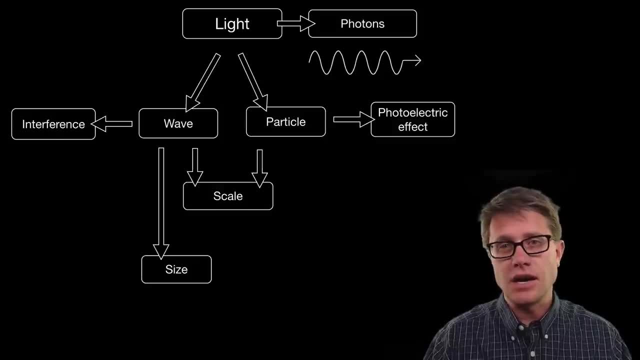 scale, And so we would use a wave model if the size of the objects that we are measuring are comparable to the wavelength of the light. And we would use the particle model if the energy that we are studying is comparable to the energy of a photon- Remember which. 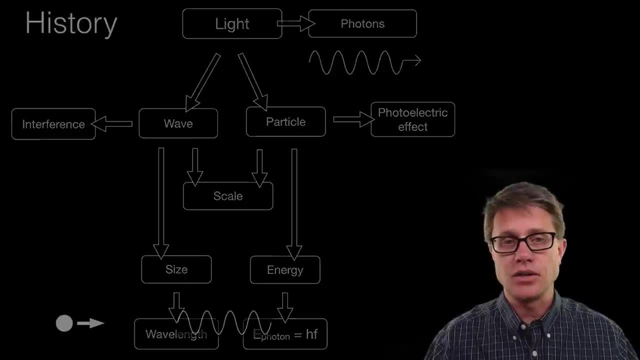 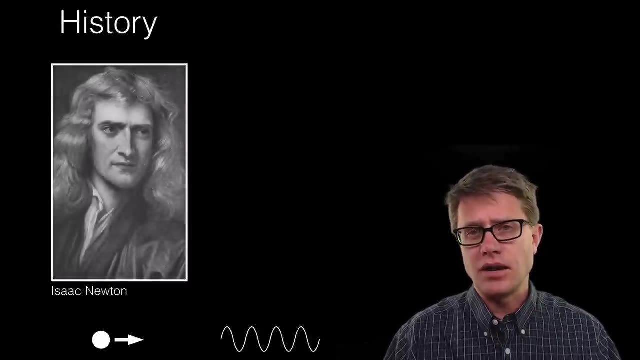 is described as Planck's constant times, the frequency of the photon itself. Let me give you a little bit of history. The first person to tackle this issue was Isaac Newton, And he thought that it traveled by the wavelength of light. And when he was trying to calculate, 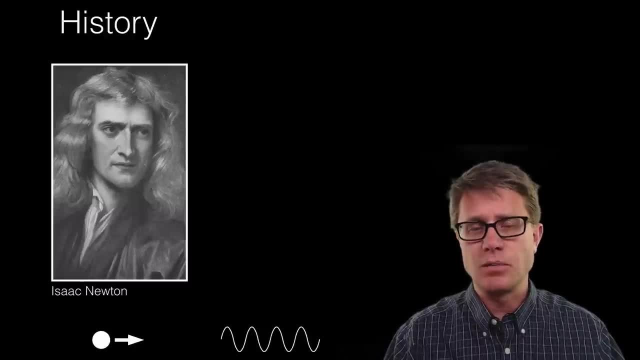 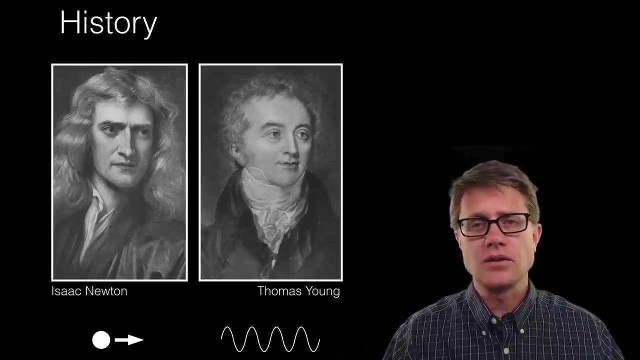 traveled in these small microscopic corpuscles or these small particles. And then finally, Thomas Young looked at that evidence, gathered more evidence and said that there are waves, And so scientists looked at this for hundreds of years. And so if we kind of look at all, 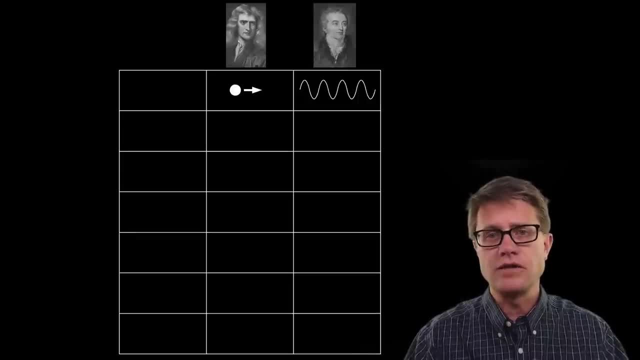 of the evidence and kind of go through those two particle and wave model. we could first start with reflection. Do they bounce off objects? And we would say yes and yes. If we look at refraction, can they bend as they move from one medium to another? We would 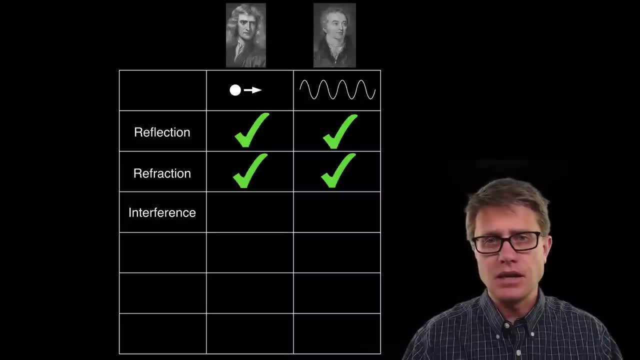 say yes and yes. If we look at interference, can they interfere with one another? The particle model does not hold up. They cannot interfere with one another, But the wave does. Do they diffract? Do they bend around objects? Or as you go through an opening, we would say: 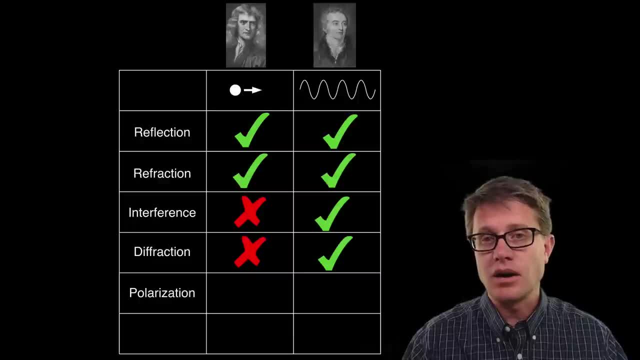 particle, no, We would say wave, yes. What about? can they be polarized, In other words when they are traveling in one dimension? can we use small slits to just limit the amount who go through? Say no And we would say yes for waves. So waves are looking great. And finally,